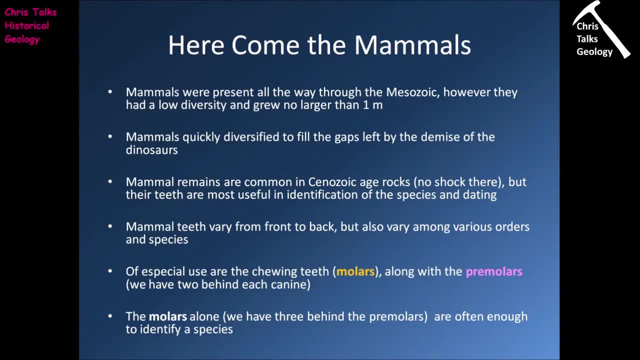 sediments and, as such, they'll become incorporated into sedimentary rocks. So, when it comes down to it, mammalian teeth in particular are exceptionally helpful for the identification of species and dating during the Cenozoic. So we know that mammal teeth vary from front to back, but they also differ. 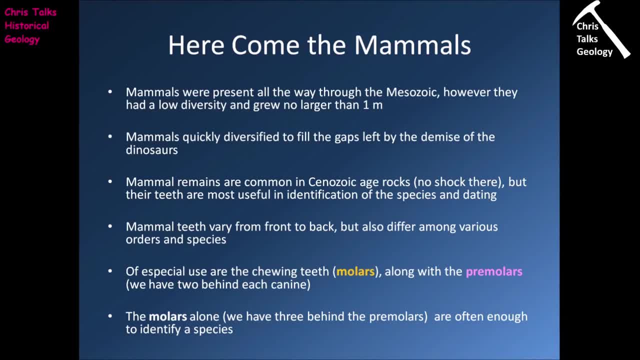 among various orders and species. So we know that one of the diagnostic features for something to be considered a mammal is the presence of differentiated teeth. So we know that mammals have incisors, canines and molars. However, the size of these teeth and the number of these teeth, they 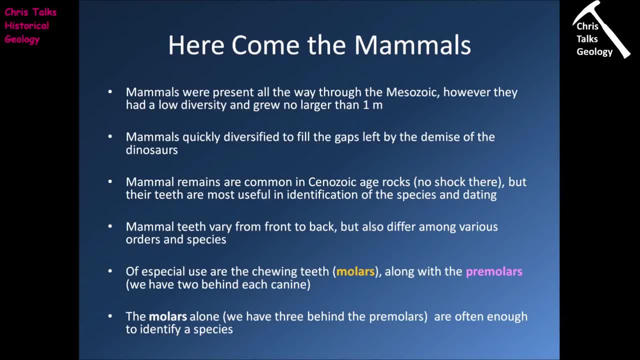 have will vary between different orders and species. So, for instance, something like the cow, obviously because it chews a lot of vegetation, will tend to have greater numbers of molars, in terms of something like a beaver, for instance. well, we know that the incisors at the front of 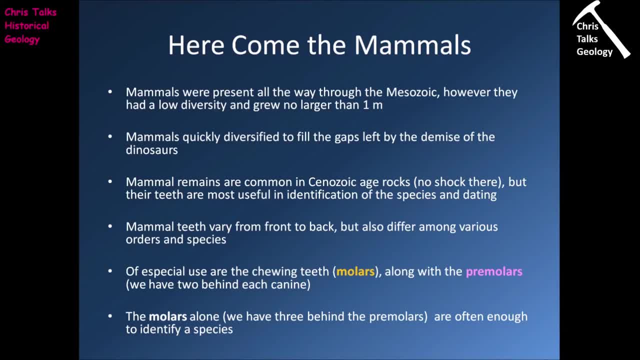 the mouth are very, very overdeveloped. Now, of a special use for identifying mammals are the chewing teeth, the molars, because they are typically the largest and therefore the hardiest teeth, and so they're more likely to survive and become incorporated into sediments. There's also 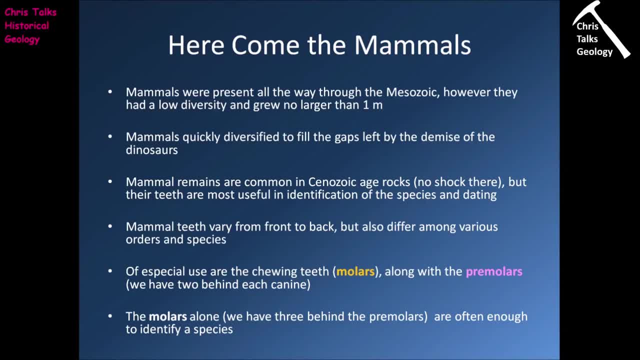 a tooth which can be useful to us. these are the pre-molars. Human beings have two pre-molars situated behind each canine and they're the teeth that kind of. they feel quite big and broad, a bit like molars, but they also have a sharper edge to them because they're designed for slicing. they're. 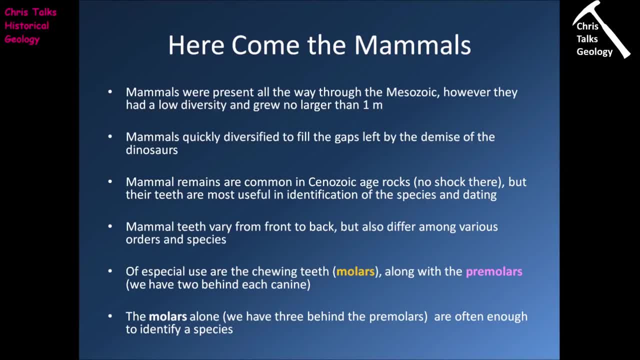 not quite designed for chewing and pulping like a true molar, they're designed for cutting up food. Now, the molars alone- of which human beings have three behind each set of pre-molars- are often enough to identify an individual species. so, as I said, they're extremely helpful when trying to identify species and date. 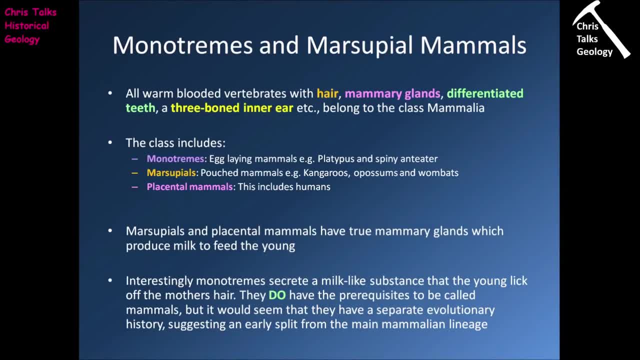 rocks from the Cenozoic. So we know that mammals are warm-blooded vertebrates that possess a range of distinct features, and some of these features include things like hair, mammary glands, differentiated teeth and a free-boned inner ear, and so all warm-blooded vertebrates that share 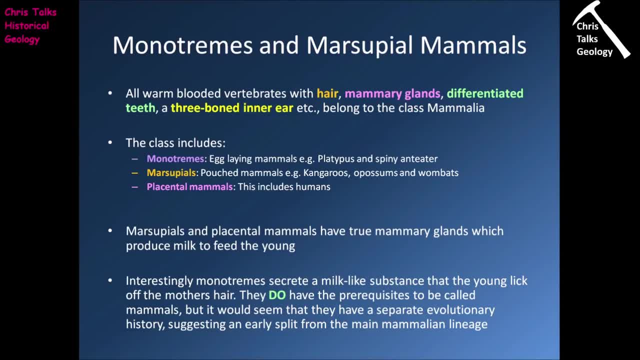 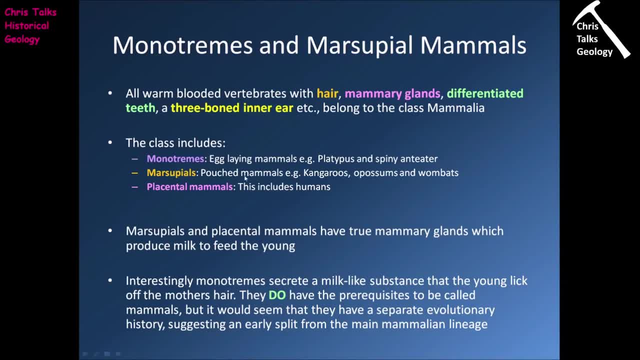 The monotremes are referred to as the egg-laying mammals, and that includes animals like the platypus and the spiny anteater. The marsupials are often referred to as the pouched mammals, and that includes organisms like kangaroos, possums and wombats, And then, finally, we have the placental. 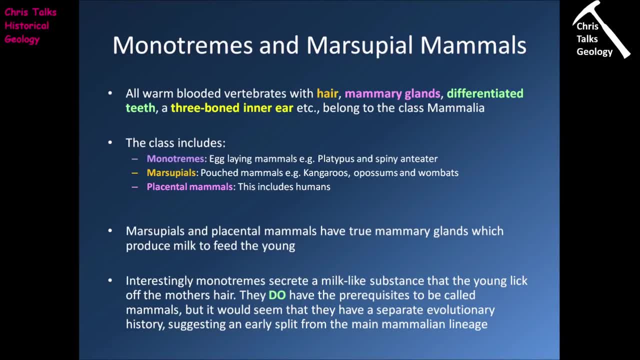 mammals, and that includes mammals such as the humans. So marsupials and placental mammals have true mammary glands which produce milk to feed the young. Interestingly though, the monotremes have developed a different method to get milk to the young, So in the case of the monotremes, the mother will secrete a milk-like substance onto her hair. 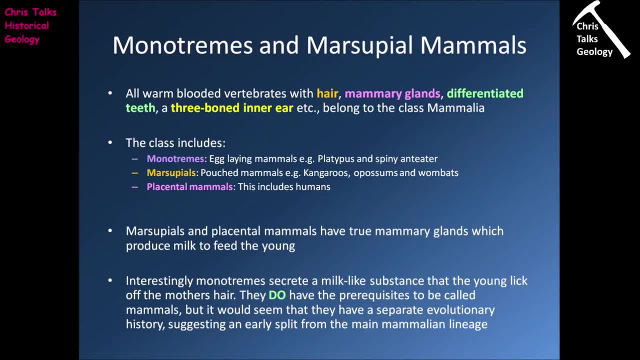 which will then be licked off by the offspring. So, to be clear, monotremes do have mammary glands and, as such, they will be considered mammals. However, there are differences and this would suggest a somewhat separate evolutionary history, and this suggests that there's a relatively early 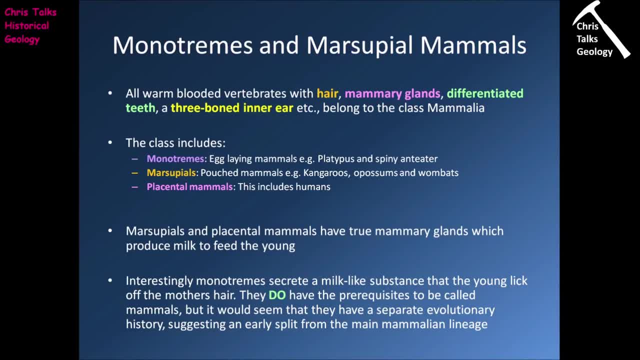 split of the monotremes from the male and the female. So there are differences and this would suggest a somewhat separate evolutionary history, and this suggests that there's a relatively early split of the monotremes from the male and the female. So there are differences and this would suggest that there's a sofort. 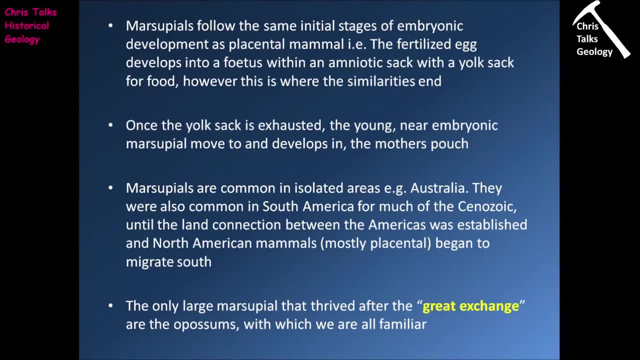 of cells produced by the m, construed to have single parts of their body. This suggests a strong link between the two groups. In the case of both groups, the fertilized egg develops into a fetus and that mother follows the same stages of embryonic development as the mother, and actuallyこれthatmies follow the same Workshop Zahlen of embryonic development as placental mammals. 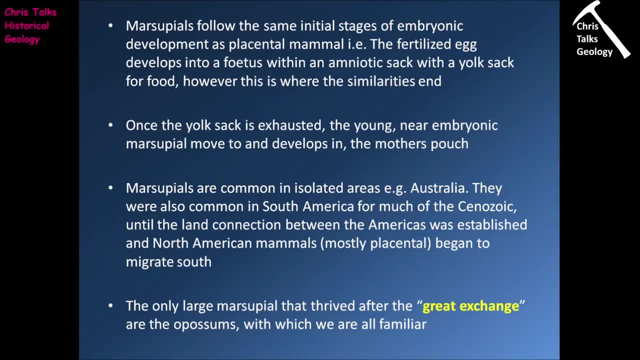 So that suggests a strong link between the two groups. So in the case of both groups the fertilized egg develops into a fetus, but also is influenced by the goodness of the encouraging male枱fet placenta and therefore is reduced to a fetus egg and is raised to a 3 million egg. 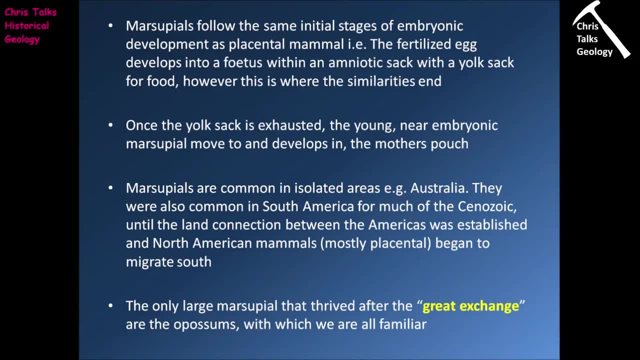 is contained within an amniotic sac with a yolk sac for food. however, this is where the similarities end In the case of the marsupials. once the yolk sac is exhausted, the young, near embryonic marsupial will then move to and develop in the mother's pouch. Now marsupials are common in 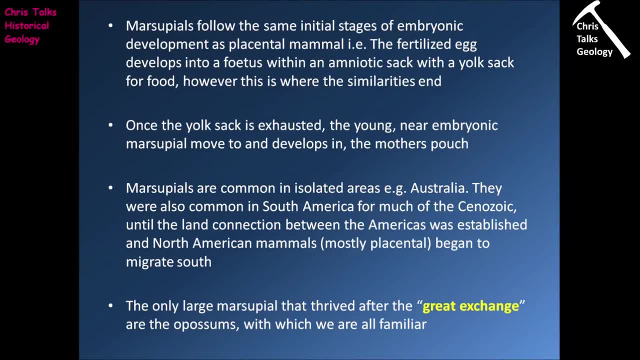 isolated areas, so somewhere like Australia. They were also common in areas including South America for much of the Cenozoic. however, that was until a land connection was made between North and South America and this allowed North American mammals, which were mostly placental mammals, to begin to. 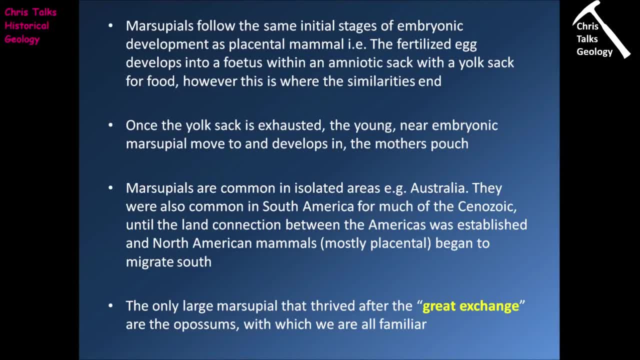 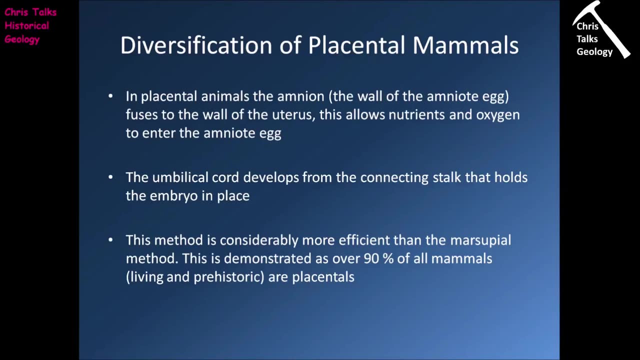 migrate south, where they began to out-compete the South American marsupials. So the only large marsupial that thrived after this great exchange, as it's sometimes referred to, were the possums, with which we're all relatively familiar. So from this point on, we're going to focus on 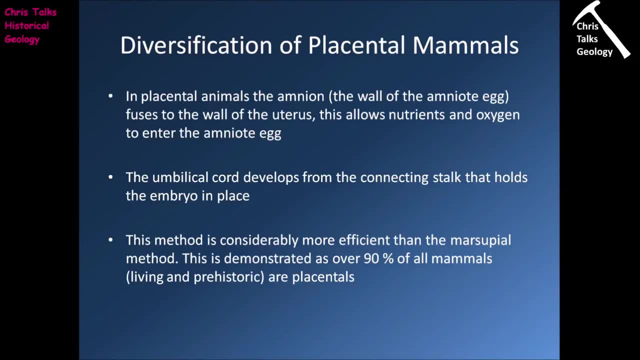 the marsupials. Now, the reason for this is that the placental mammals make up over 90% of all mammals, both living and prehistoric, so they're by far and away the most successful group. This means they are also going to be the most numerous group of mammals in the Cenozoic and, as such, they're going to show the 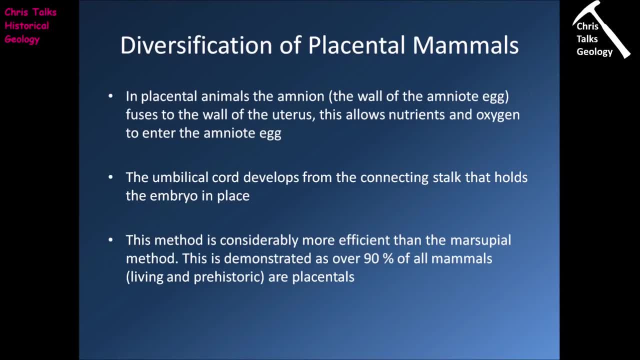 most evolutionary diversification, and so it's not really surprising that we're going to want to really focus in on them and see what was happening Now. placental mammals differ from the marsupials in the method of embryonic development, So there are similarities in the initial stages. So, as we've discussed both groups- 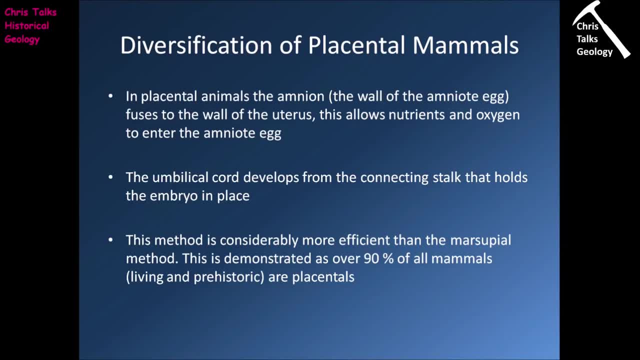 the marsupials and the mammals produce amniote eggs when within that amniote egg there is a yolk sack that supplies food to the embryo, initially. Now, in the case of the marsupials, once the yolk is exhausted, the juvenile marsupial will then migrate to a pouch in which it will develop. In the case of the placental, 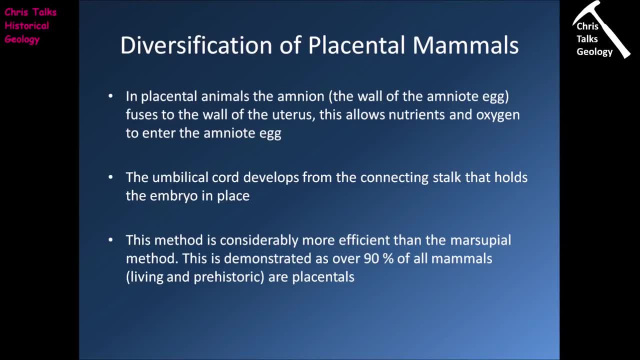 mammals. what will happen is that they will develop a certain amount of eczema, such as a lot of the is the amnion, which is the wall of the amniote egg, will fuse to the wall of the uterus, and this will allow an exchange of nutrients and oxygen between the mother and the amniote egg. On top of 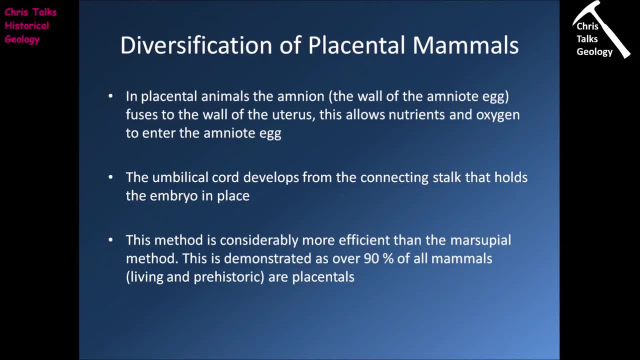 this, we're also going to see the development of an umbilical cord which will connect the embryo to the mother. Now the umbilical cord is going to form from a connecting stalk which is part of the amniote egg, and the connecting stalk is designed, at least initially, to hold the embryo in place. 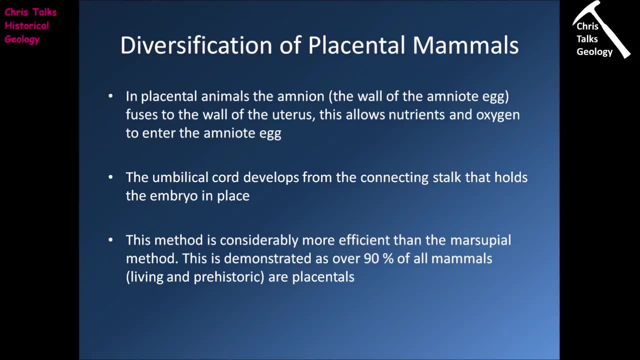 inside the amniote egg. So what we can see is that, on the whole, the placental mammal method of reproduction is more efficient than the methods used by the monotremes or the marsupials, and so this helps to explain the dominance of the placental mammals over the other two subgroups. 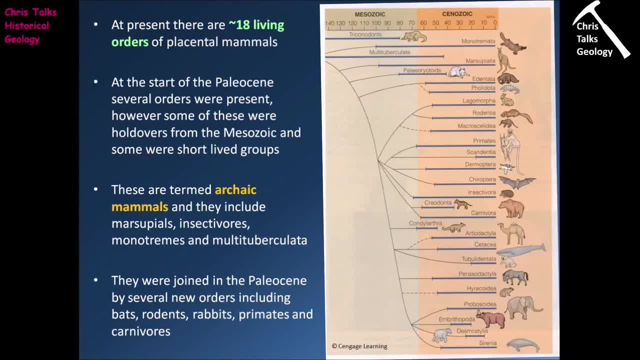 in the class mammalia. So at present there are approximately 18 living orders on the amniote egg and the placental mammal method of reproduction. So this helps to explain the dominance of the placental mammals over the other two subgroups in the class mammalia. 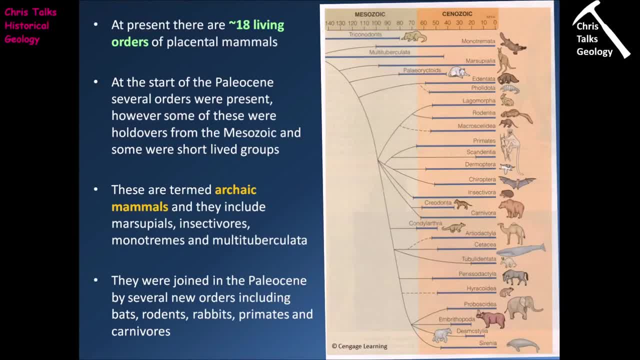 Now at the start of the Paleocene, so that's the start of the Cenozoic. we had several orders of placental mammals that were present. however, some of those were holdovers from the Mesozoic and some were relatively short-lived groups. Now, these placental mammals which made their first appearance, 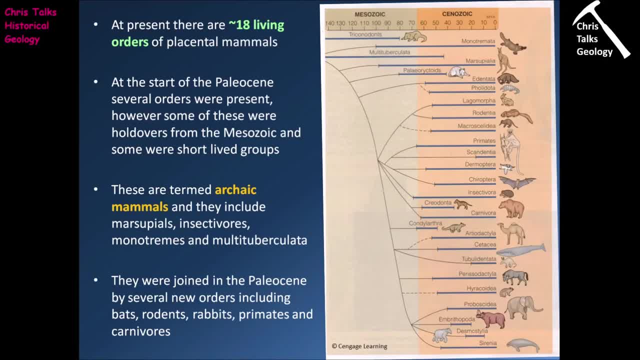 in the Mesozoic and continued over into the Cenozoic are termed the archaic mammals, and they include groups like the marsupials, the insectivores, the monotremes and the multituberculata. Now, they were then joined in the Paleocene by several new orders of placental. 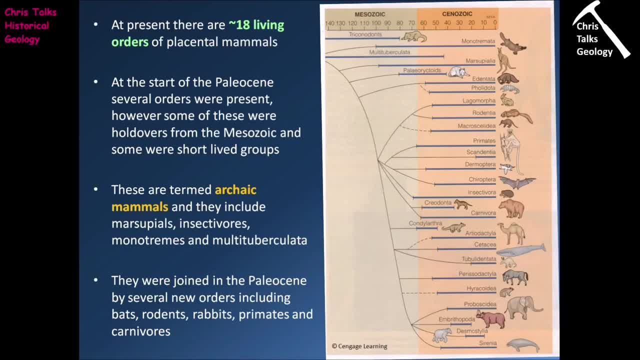 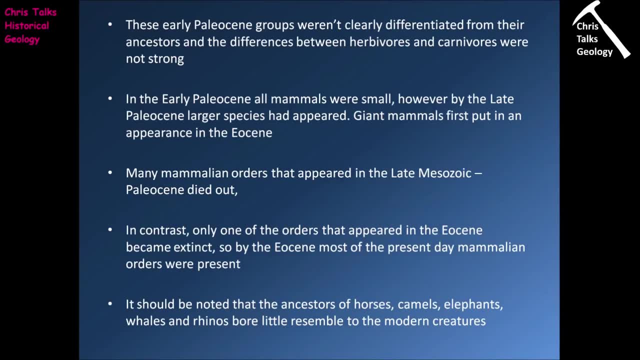 mammals, including the bats, the rodents, the rabbits, the primates and the carnivores. So these early Paleocene groups of placental mammals weren't clearly differentiated from their ancestors and the difference between herbivores and carnivores weren't particularly strong. and of course this makes sense because in the early Cenozoic we were in the early stages of. 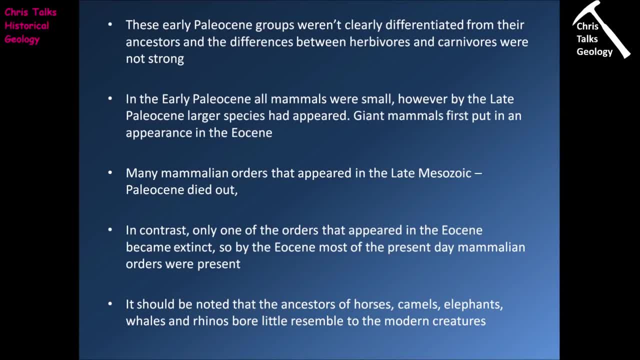 mammalian divergence, and so there's going to be quite a few similarities between individual groups. Now, in the early Paleocene, most mammals would have been small. however, by the late Paleocene we begin to see the evolution of larger body designs. We don't see the appearance of the giant. 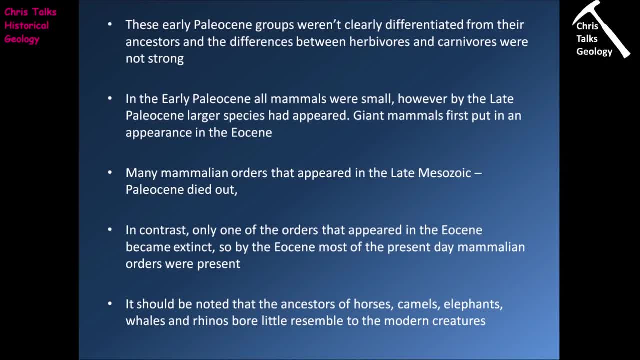 mammals until the Eocene. and of course this makes sense for two reasons. Number one, it's obviously going to take time for evolution to produce very large body designs. and number two, it's going to in the early Cenozoic there's also going to be competition from larger bird species. and of course, 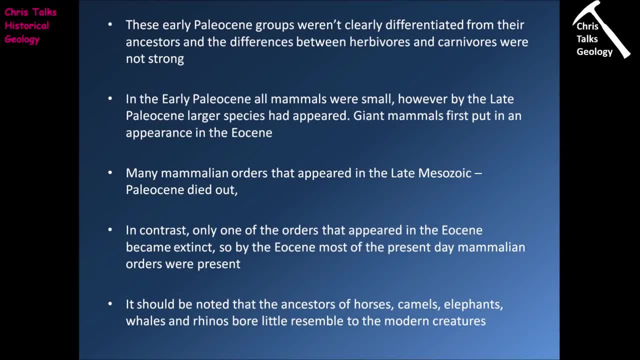 this is going to mean that it takes a little bit longer for larger mammalian species to begin to evolve and out-compete those larger bird species. Now, many mammalian orders that appeared in the late Mesozoic to early Paleocene went and died out. so they were designed for the time. but as 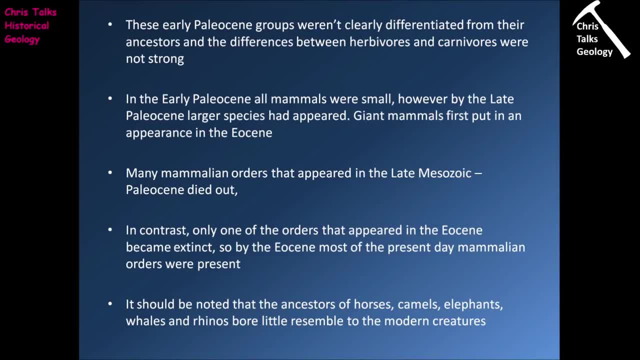 evolution begins to move forward, they very quickly find themselves becoming out-competed by the more advanced mammalian groups. In contrast, only one order that made its appearance in the Eocene became extinct. so by the Eocene most of the present-day mammalian orders were represented. 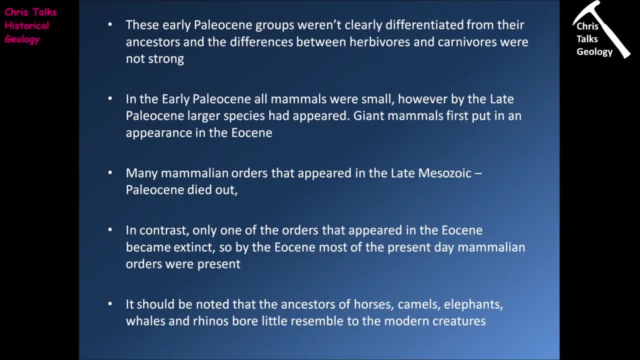 Now. it should be noted, though, that of the present-day mammalian orders, groups like the horses, the camels, the elephants, the whales and the rhinos bore little resemblance to modern-day creatures, so there's still quite a lot of evolution yet to be done. So the warm, humid North American. 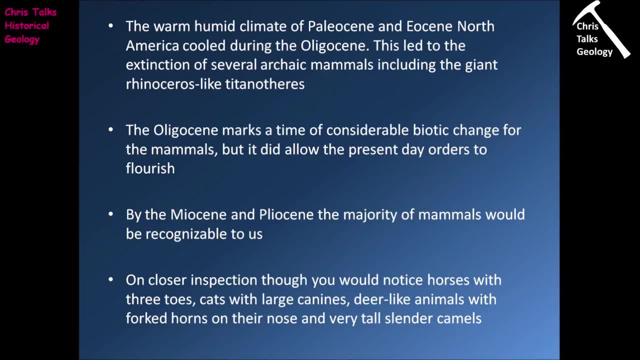 season of the Paleocene and Eocene cooled during the Oligocene and of course this cooling is going to bring about extinction. so it leads to the extinction of several groups of placental mammals, including the giant rhinoceros-like Titanotheres. Now the Oligocene marks a time of considerable. 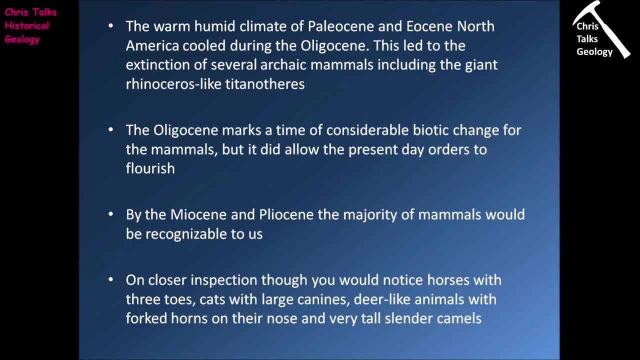 biotic change for the mammals, but it did allow the present-day orders to establish themselves and flourish Now by the Miocene and Pliocene. the majority of mammals would be recognizable to us. however, on closer inspection we would notice differences. so, for instance, we would see things. 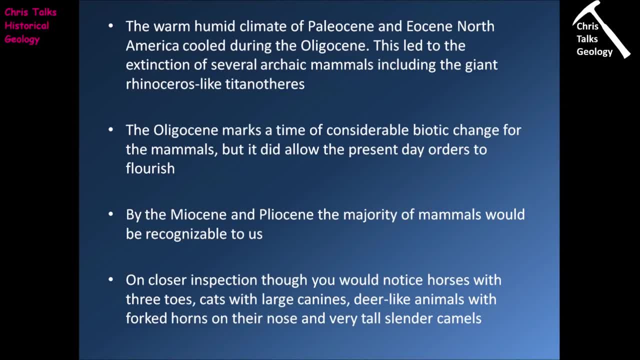 like horses that had free toes, cats that had very oversized canines, deer-like animals that had forked horns on their noses and things like tall, slender camels. So although we could recognize what we were looking at, we would see there were still significant differences. 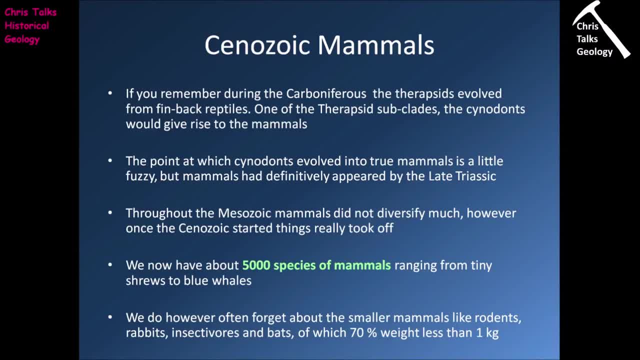 So now let's move on to focus on individual groups of mammals. during the Cenozoic- Now, if you remember, during the Carboniferous, so that's the Paleozoic- the Therapsids, which were a group of mammalian-like reptiles, evolved from a group of thin back reptiles called the Plycosaurs. 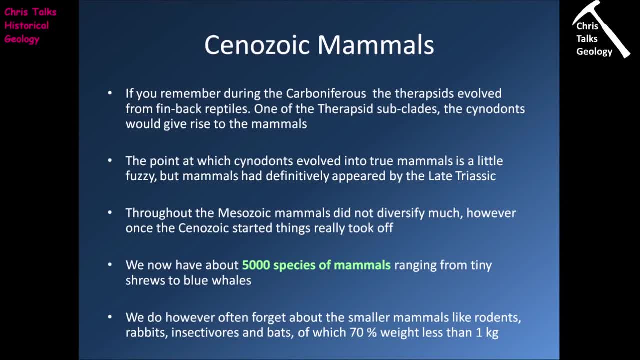 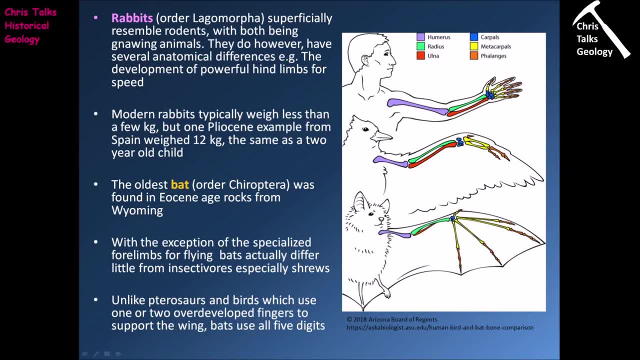 evolved from a group of thin back reptiles called the Plycosaurs. Now one of the Cynodonts evolved from a group of thin back reptiles called the Plycosaurs. Now one of the Cynodonts actually use all five digits to support the wing membrane. you can actually see that over here. 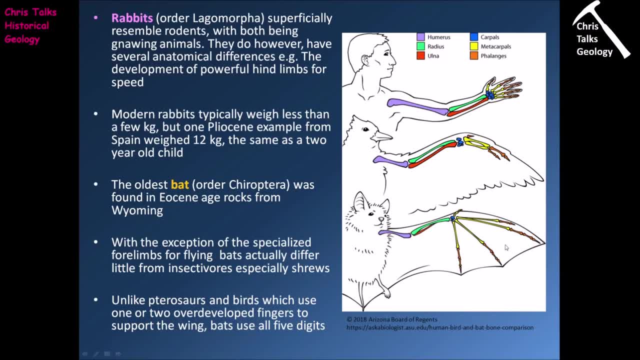 you can see how the bat forelimb is designed to use all five fingers in order to keep the wing membrane taut to allow for flight. compare that to the bird, where you can see the wing is primarily being supported by simply two digits. the other thing you can quite clearly see once again is: 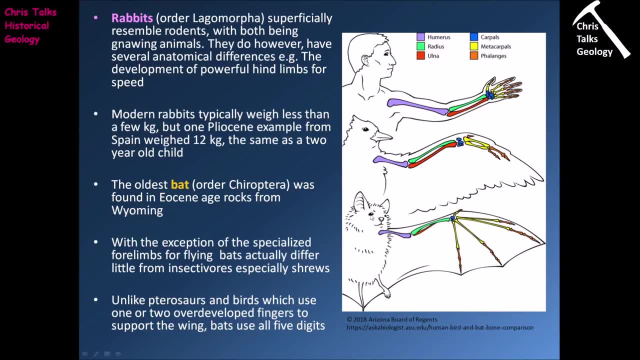 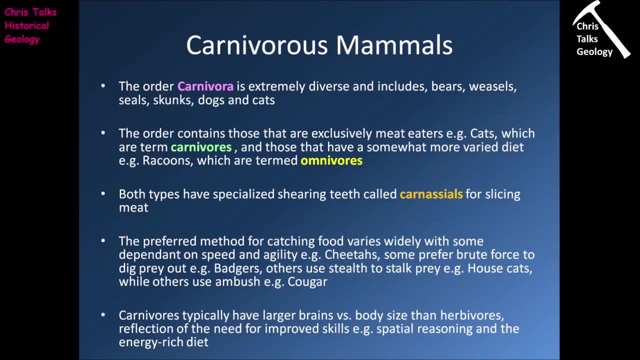 the similarity between the forelimb designed for groups like humans, birds and bats, which of course, show that we all have a common ancestor. so now let's move on to the carnivorous mammals. so the order carnivora is extremely diverse. it includes organisms like bears, weasels, seals, skunks. 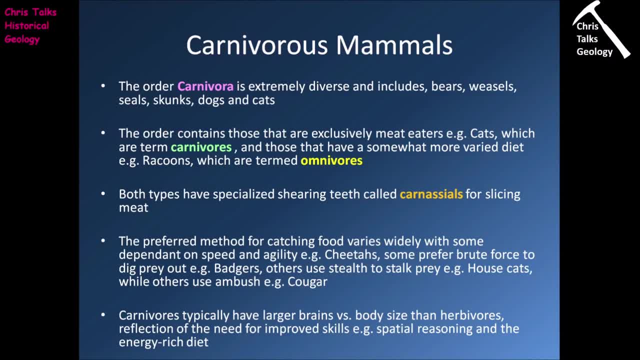 dogs, cats, etc. now the order contains those mammals which are exclusively meat eaters, so that would be something like a cat, for instance, which we term carnivores. but it also contains organisms which have a more varied diet, so something like a, and that is going to include animals which are termed omnivores, so they will consume both meat. 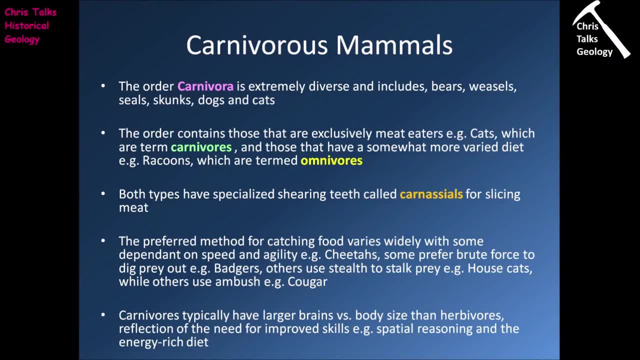 and plant material. So both types of carnivorous mammals, so that's the carnivores and the omnivores, have specialized shearing teeth called carnassials, and these are designed for slicing meat and they're situated before the molars, on the lower jaw of carnivores. Now these teeth are a key diagnostic. 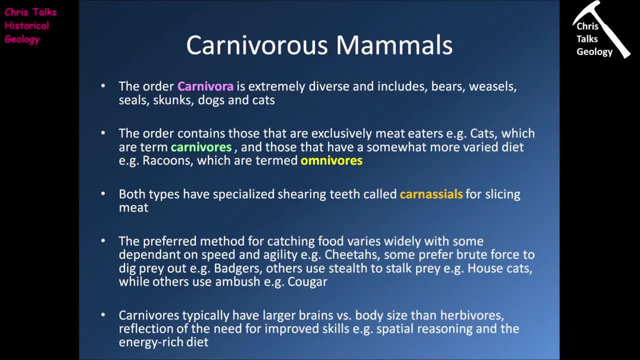 feature for something to be considered part of the order carnivora. Now, the preferred method for catching food varies widely within this group, with some carnivores being dependent on speed and agility, so a good example would be a cheetah. Some prefer more brute force techniques to get to. 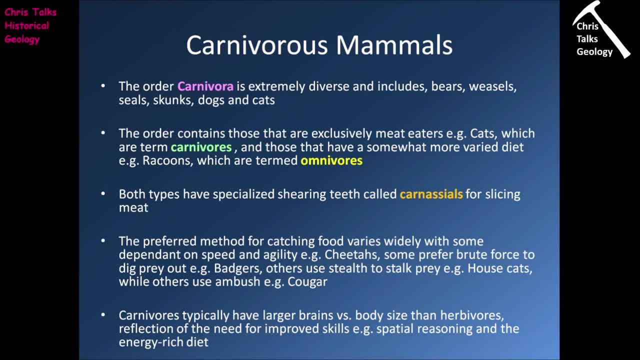 their prey, so that would be something like a badger. Others prefer to use stealth to stalk their prey, so that would be in groups like house cats, while others are ambush predators like cougars. Now, carnivores typically have quite a large brain to body size ratio, and it's typically much. 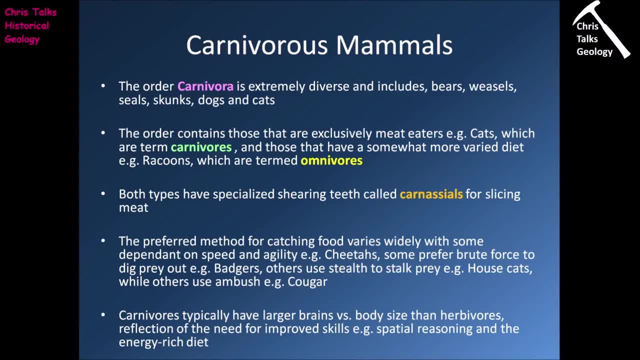 greater than that of herbivores, and this is a reflection of the need of carnivores to have an improved skill set, so they have to have better spatial reasoning, for instance when compared to a herbivore, because it's advantageous when hunting, but it's also a reflection of their more energy. 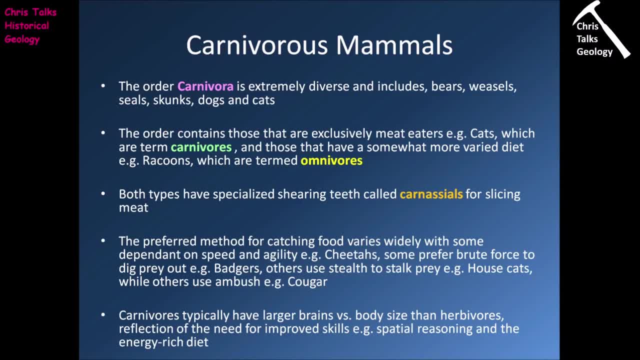 rich diet, so meat offers a much richer energy source and, of course, this means they can therefore support their prey. So if you're a carnivore and you're a carnivore, and you're a carnivore and you're the high energy requirements of a large brain, So when we look at the fossil record for cenozoic, 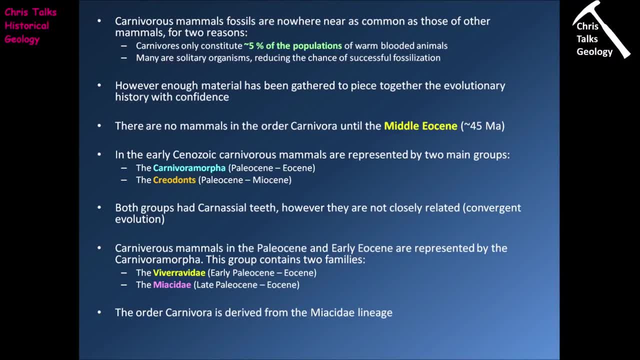 carnivorous mammals, we see that they're nowhere near as common as fossils of other mammalian groups. Now, there are two reasons for this. The first one is that carnivores only constitute approximately five percent of the population of warm-blooded animals. Now we've already covered. 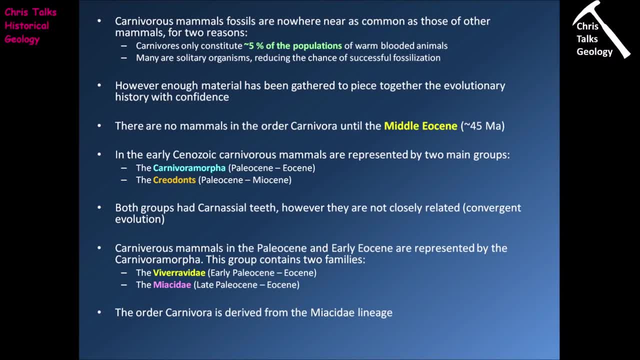 this is that when animals are warm-blooded, obviously they have a higher metabolism, and this means they require more food in order to function, and so that means, in order to support a population of warm-blooded predators, you need to have a very plentiful food source, so you need to have lots of 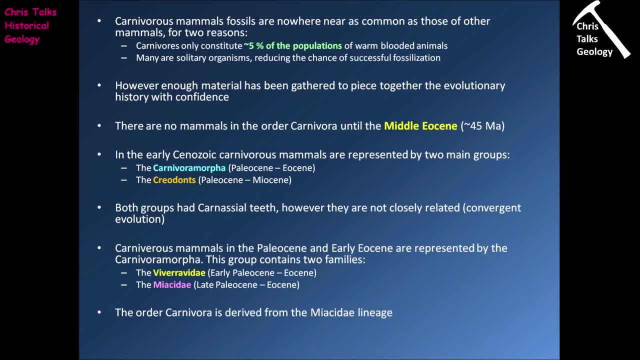 prey animals on which those warm-blooded carnivores can feed, and so this obviously means warm-blooded carnivores can only constitute a small percentage of the overall population. Now, the other reason that carnivorous mammal fossils are relatively rare is that, on the whole, they're quite solitary. 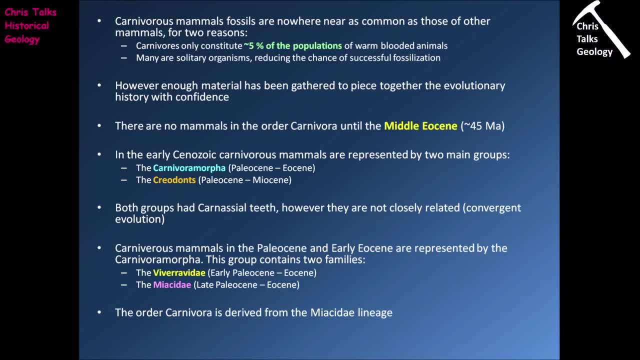 organisms, and this reduces the chances that they will successfully fossilize. However, we do have enough material from the cenozoic to allow us to piece together the evolutionary history of the carnivorous mammals with a reasonable degree of confidence. So to be clear, there are no mammals. 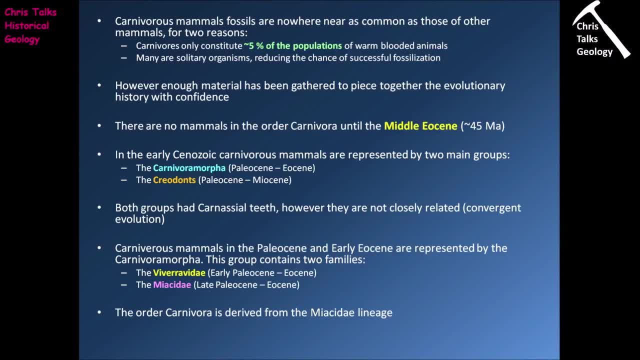 in the order carnivora until the middle ear scene, so approximately 45 million years ago. Now, this means in the early cenozoic, carnivorous mammals are represented by two main groups. there's the carnivora morpha and the creodonts. So the carnivora morpha make their 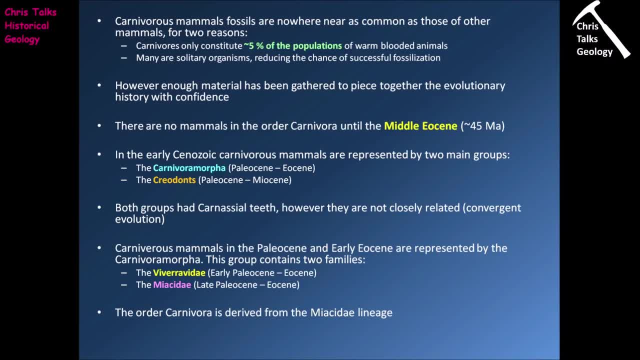 appearance in the paleocene and they go through to the ear scene. The creodonts make their appearance in the paleocene and they go through to the myocene. To be clear, the carnivora are going to evolve from the carnivora morpha. 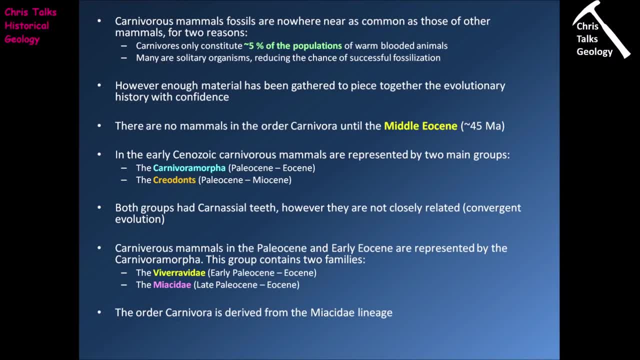 Now both groups, the carnivora morpha and the creodonts, have carnaceal teeth. however, they are not actually closely related. So this is an example of convergent evolution, where we have similar biological structures appearing in animals that have completely different evolutionary lineages- Now the carnivorous mammals- so that's the carnivora morpha- which make their appearance. 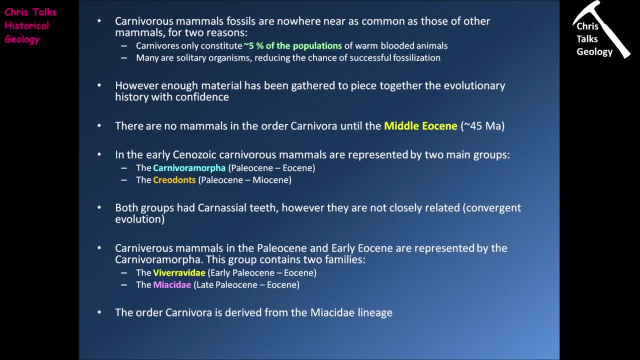 in the paleocene and go through to the early ear scene. Now the carnivorous mammals are represented by two families: there's the vivaravidae and the myosidae. Now the vivaravidae make their appearance in the early paleocene and they go through to the ear. 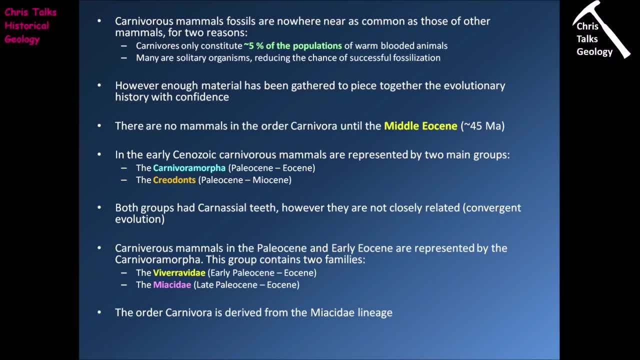 scene, at which point they become extinct. Now the myosidae also go from the late paleocene through to the ear scene, but they are the lineage which is then going to give rise to the order carnivora. and once the order carnivora are established, they're then going to begin to diverge from the 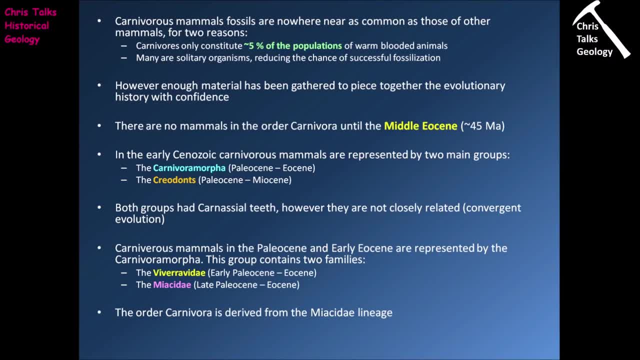 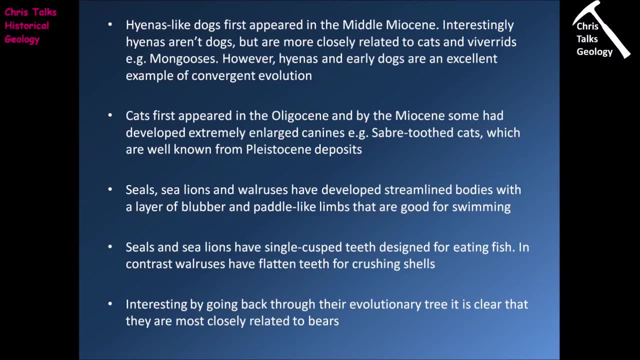 origin and that's eventually going to result in the evolution of the carnivorous mammal groups with which we are familiar today. So once we have the order carnivora established, we begin to see divergence and the appearance of certain key carnivorous mammal body designs and carnivorous 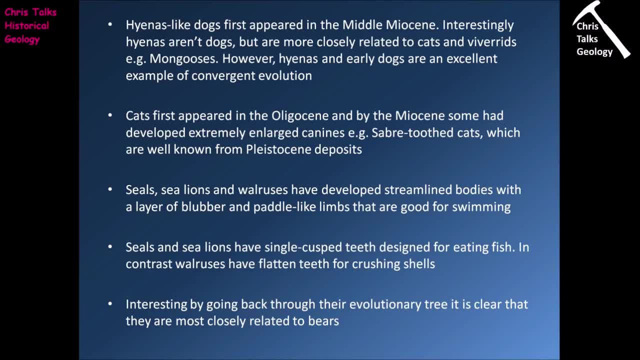 mammal groups. So, for instance, we begin to see the appearance of hyena-like dogs in the middle myosene, although, interestingly, hyenas aren't related to dogs, They're more closely related to cats and the group which we call the vivarids, that's a group that 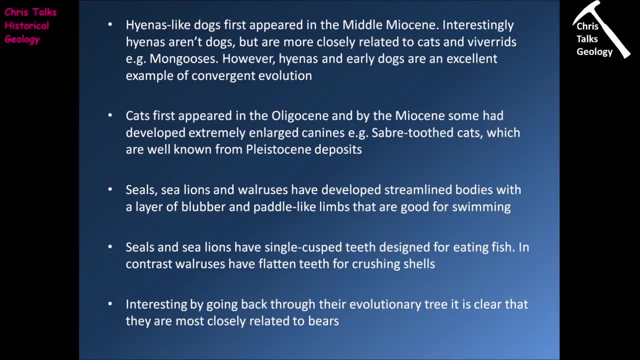 includes mongooses. However, hyenas and early dogs are an excellent example of convergent evolution. so of course that's the a similar body design occurring for animals which have completely different evolutionary lineages. We see the first cats appearing in the oligocene and by the myosene. 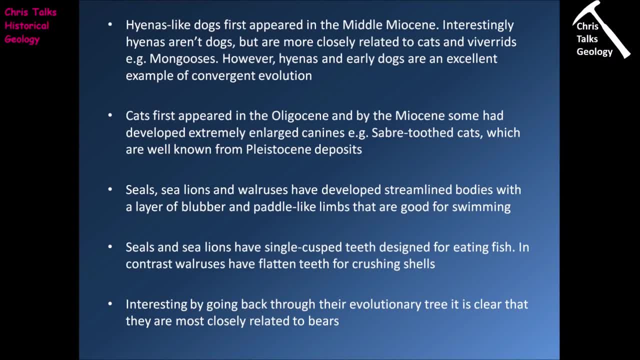 we have the development of some cat species with extremely large canines and of course, this lineage is going to be the first to appear in the early paleocene. So we're going to see the evolution of the sabre-toothed cats, which are well known from Pleistocene deposits. 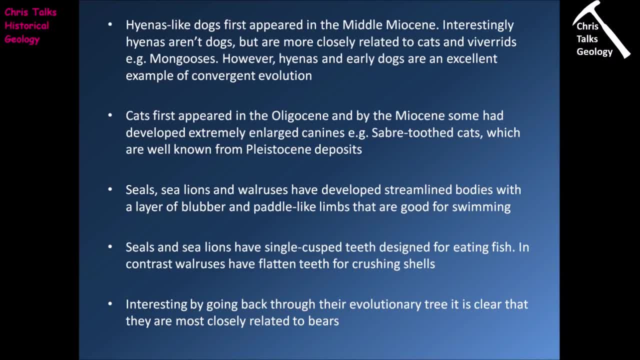 We also begin to see the appearance, or evolutionary trend, should I say, which is going to give rise to the seals, sea lions and walruses. We see their adaptation to the marine environment beginning. so we see the evolution of streamlined bodies with a layer of blubber and the evolution of